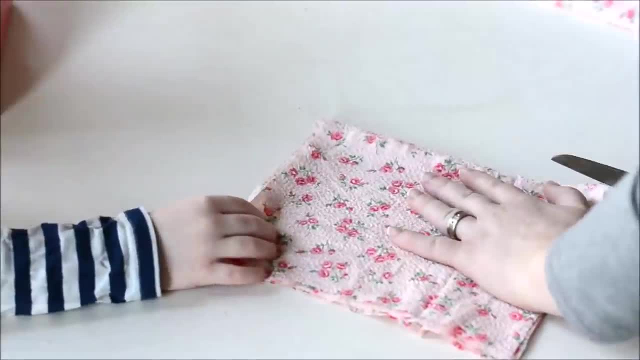 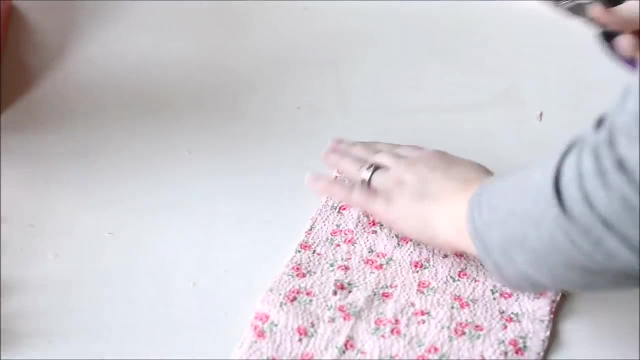 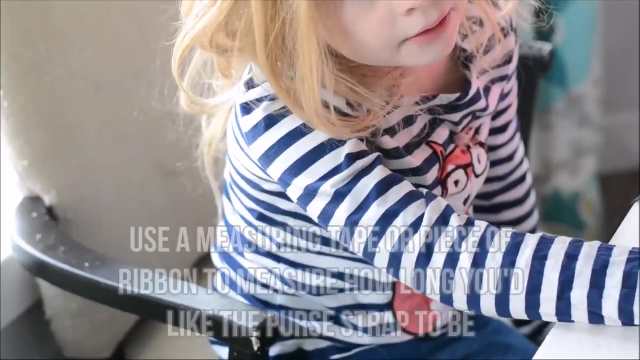 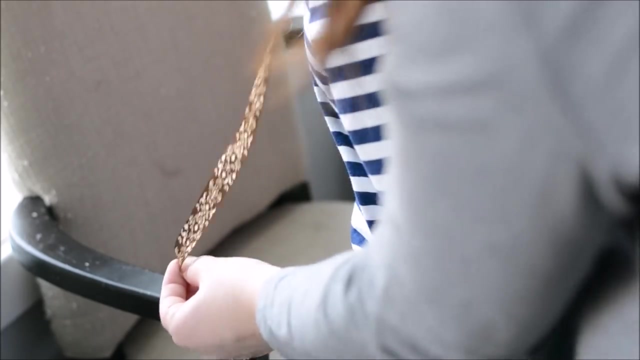 of fabric. Use a measuring tape or a piece of ribbon to measure how long you'd like the purse strap to be. So grab your model, stick the measuring tape or the ribbon over their shoulder and use that as a guide. Then lay this down onto your 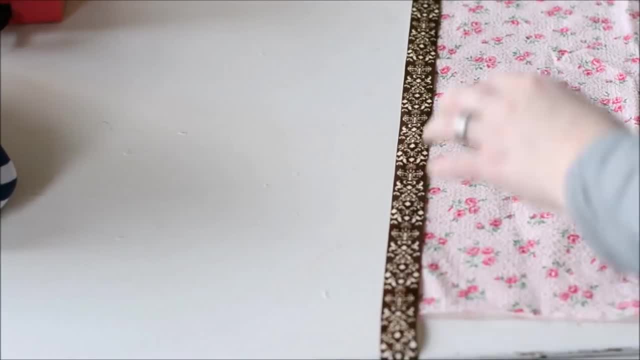 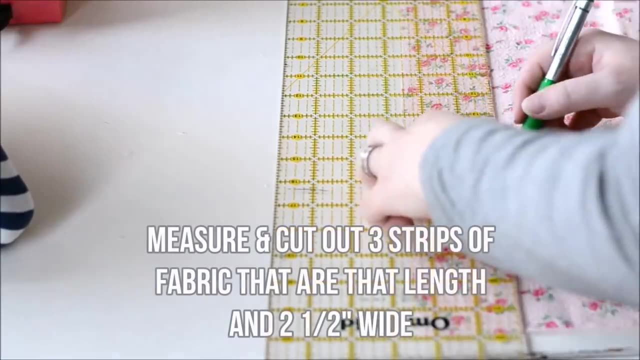 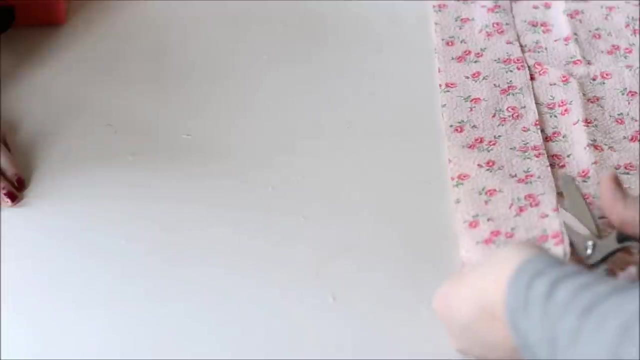 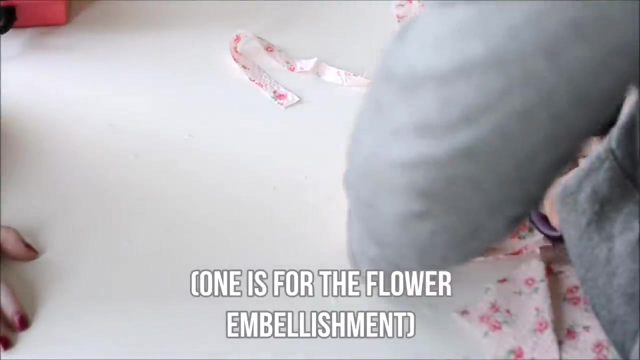 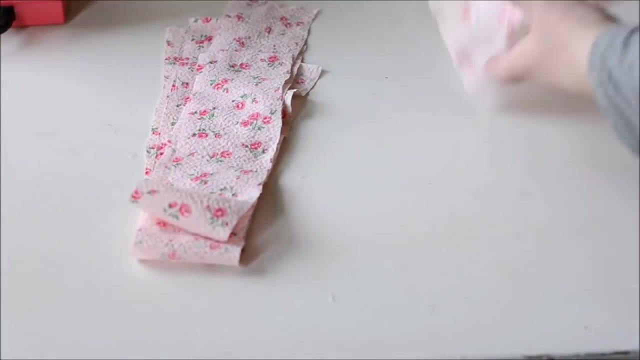 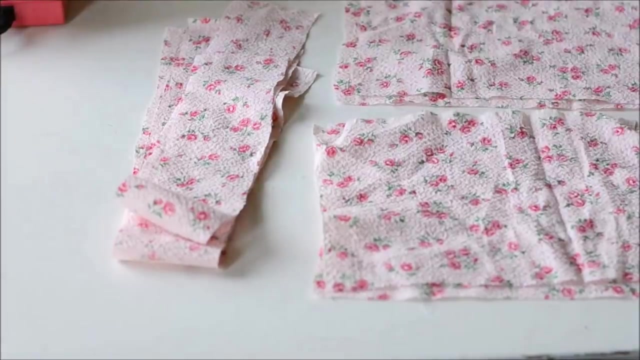 fabric to determine the length of your strap pieces. Using that hard ruler, again measure and cut out three strips of fabric that are that length and two and a half inches wide. One of these strips is going to be for the flower embellishment Place. two of 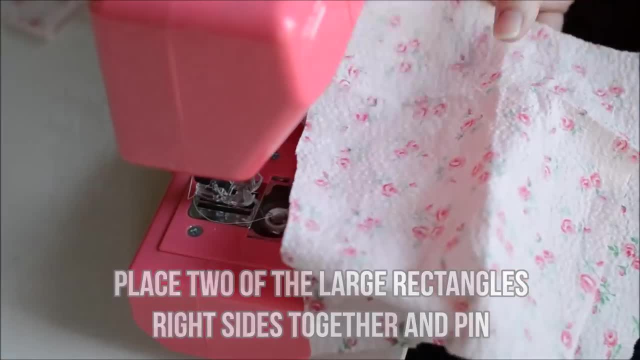 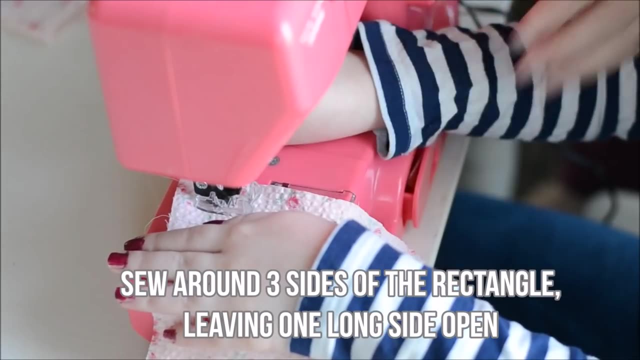 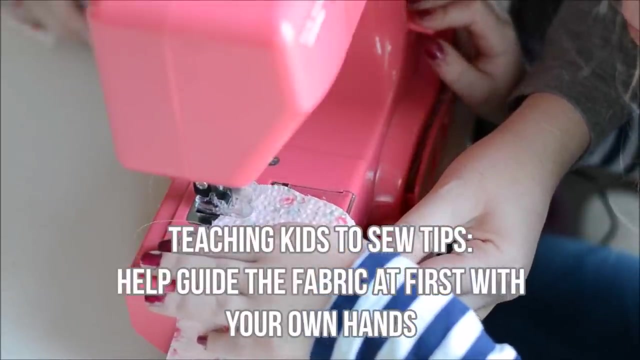 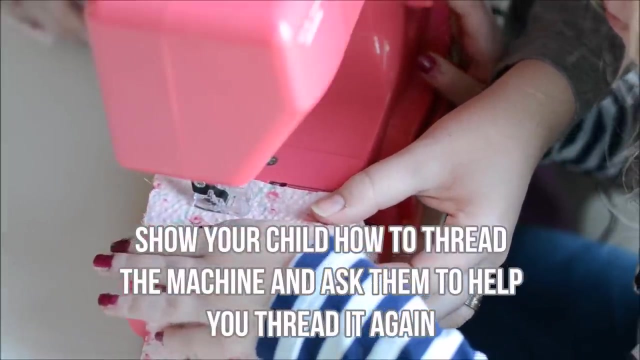 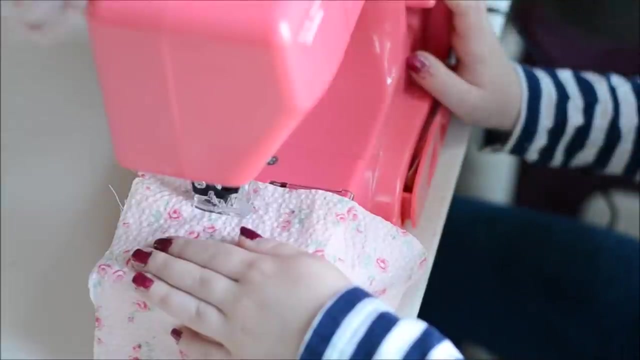 the large rectangles of right sides together and pin Here. we didn't pin, but really you should. It'll make it a little bit easier to pin. You also don't need a glue gun. if you don't have one, Just make sure you don't. 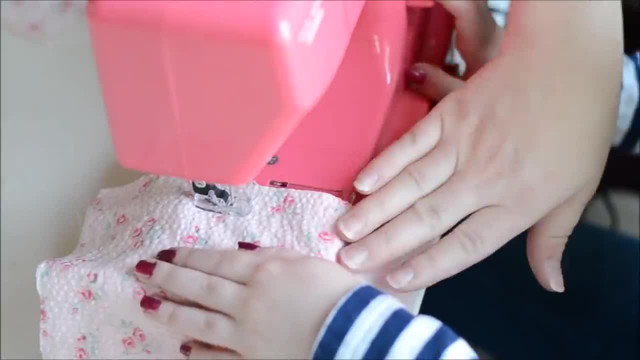 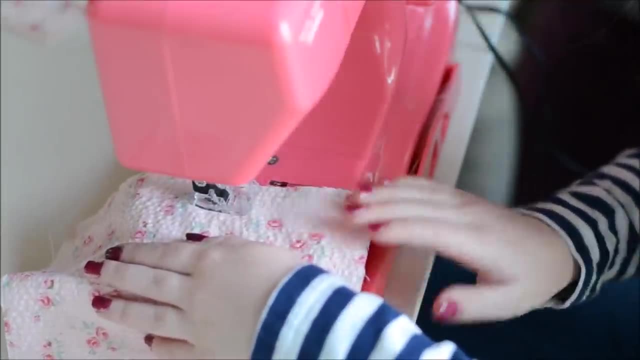 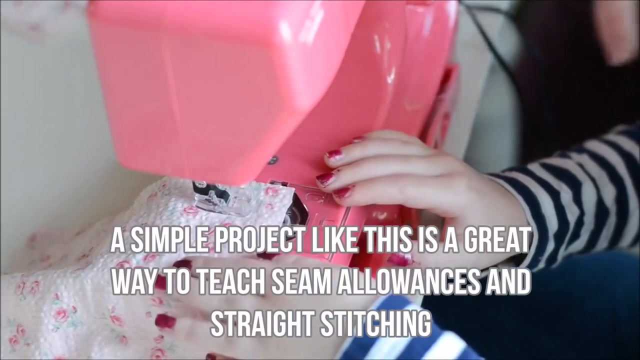 know me and I will put a link to it in the description box below. Guide your child's hands as they sew and encourage them to stop the machine whenever needed. Make sure to let them know that they can stop and start again whenever they need to. A simple project like this purse is a really great way to teach seam. 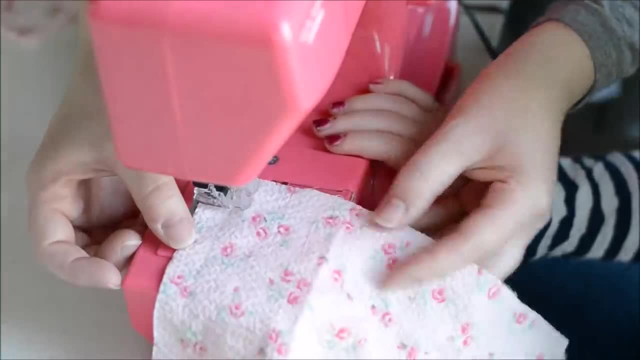 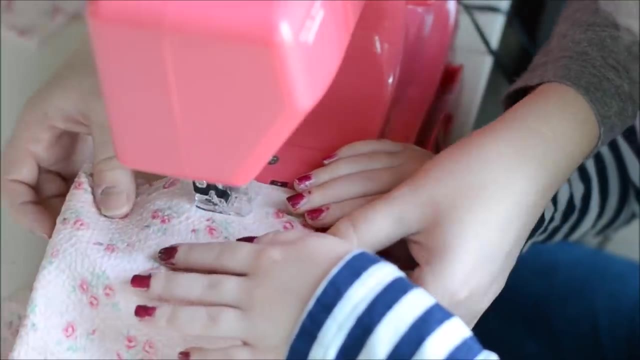 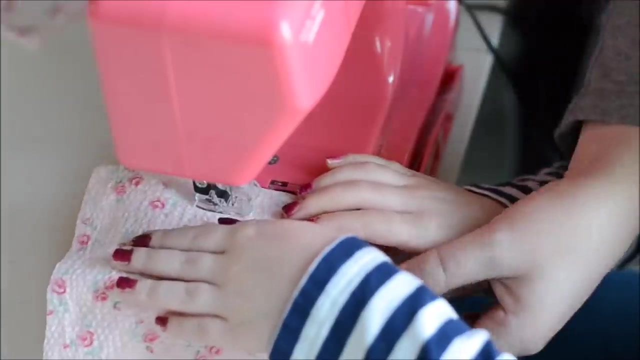 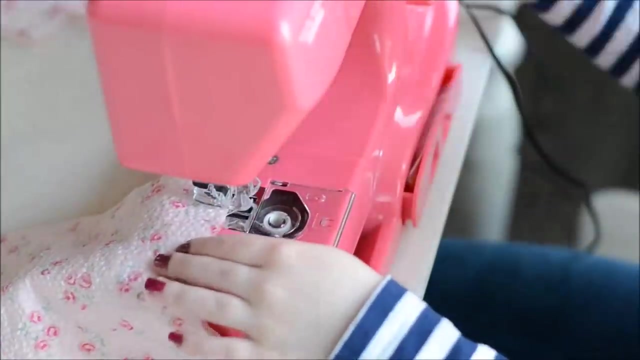 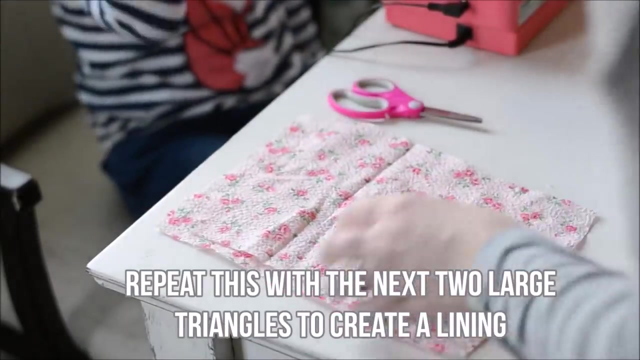 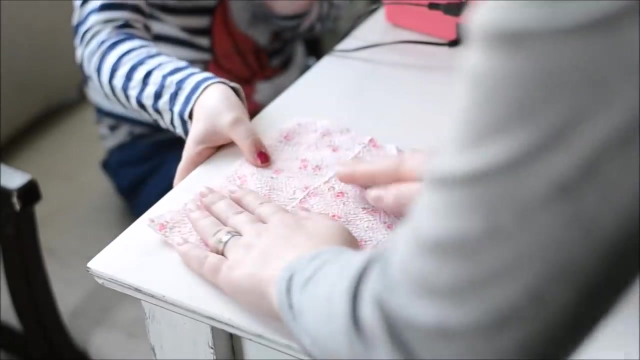 allowances and straight stitching to your child. So something like this that just involves lots of straight lines and pivoting and square sewing is just a perfect project for them to begin Now. repeat this with the next two large triangles to create a lining piece. So you're going to put them right sides together and then have your child sew. 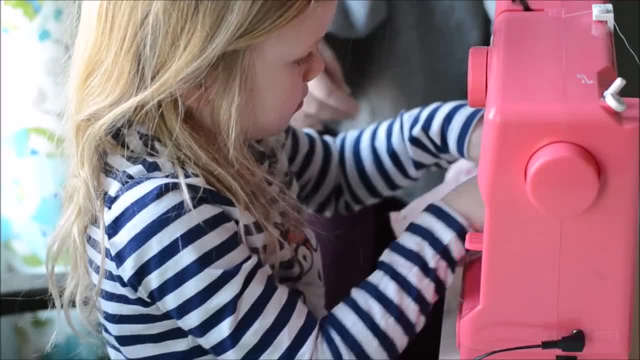 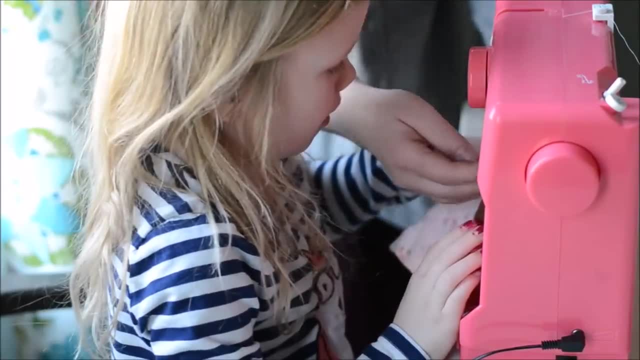 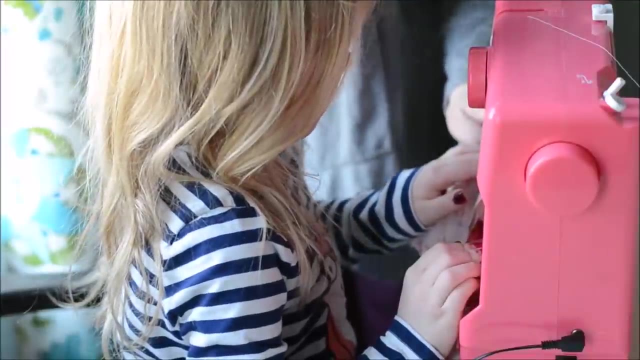 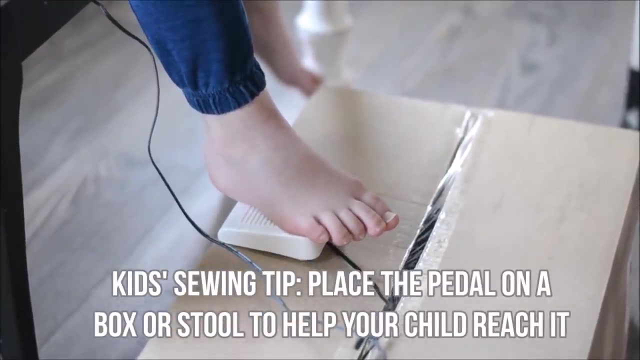 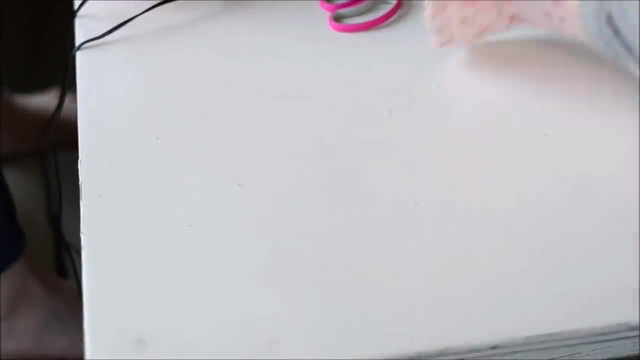 around. Here's another kids sewing tip. Place the petal on a box or a stool to help your child reach it better. Clip all of the corners of the bag pieces And then turn one of them right side out, making sure to push out those corners so. 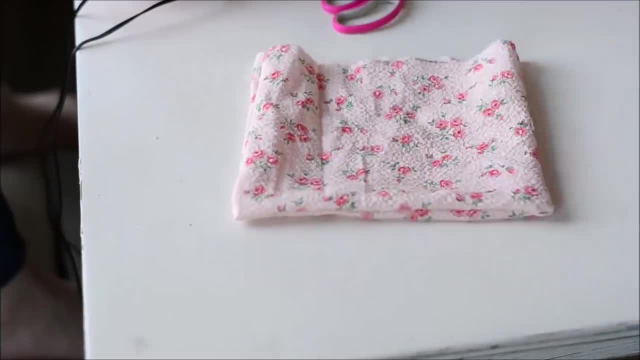 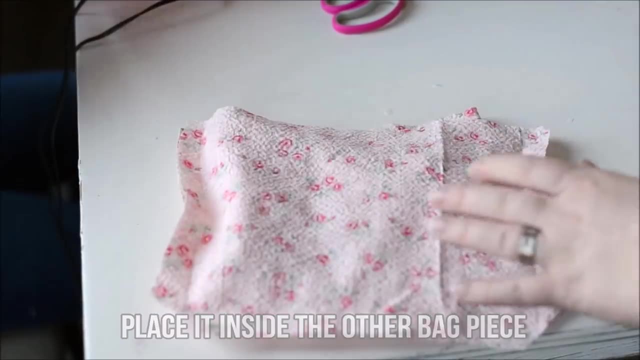 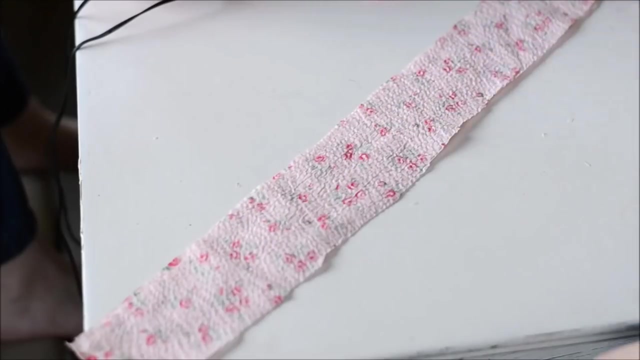 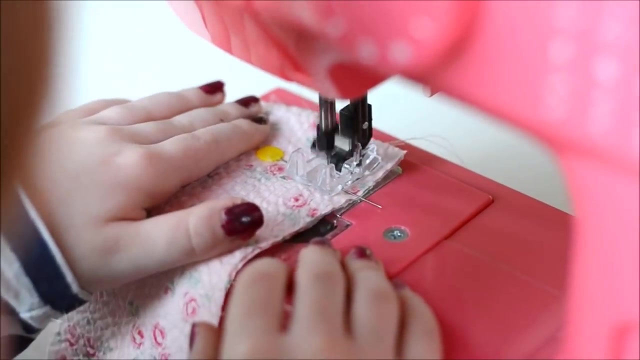 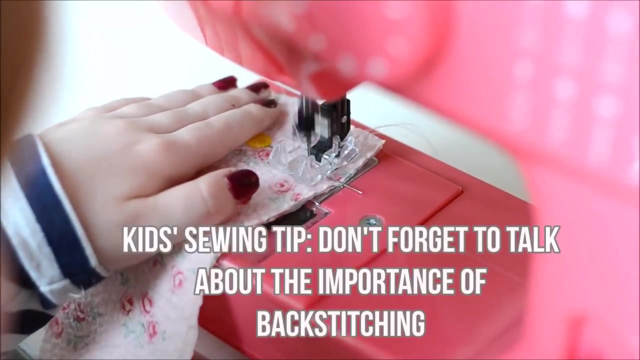 they're nice and even Place this one inside the other bag piece. Next, place the two handle pieces right sides together and pin. Now you're going to sew along both long sides of that strap with a half inch seam allowance. Here's another kid sewing tip. Don't forget to talk about the importance of 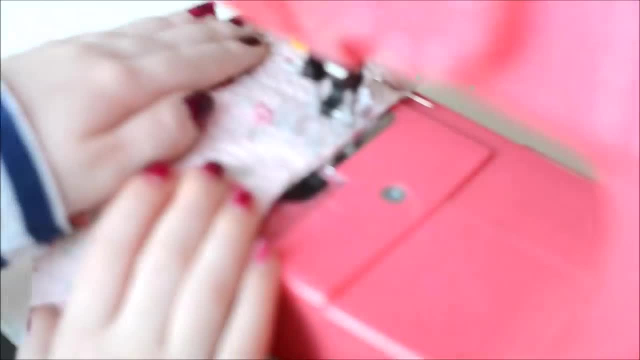 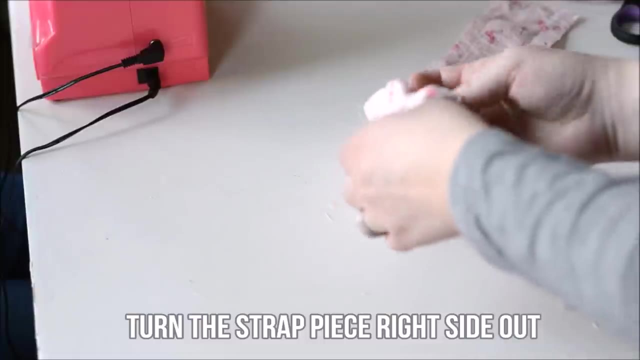 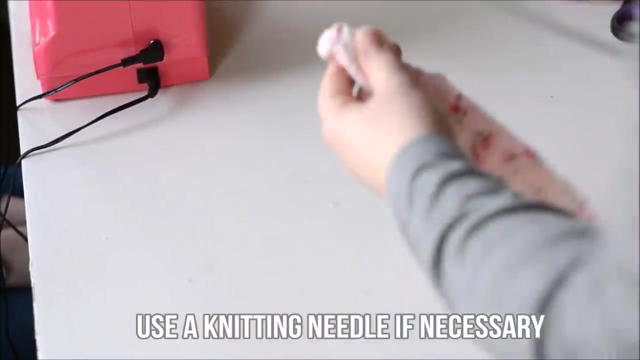 backstitching at the beginning and the end of each seam. Now turn the strap piece right side out. You can use the help of a knitting needle if you need to. Now you're going to make your return to the home. This is your return to home. 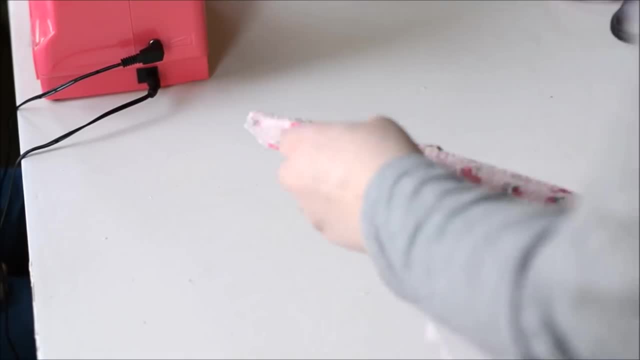 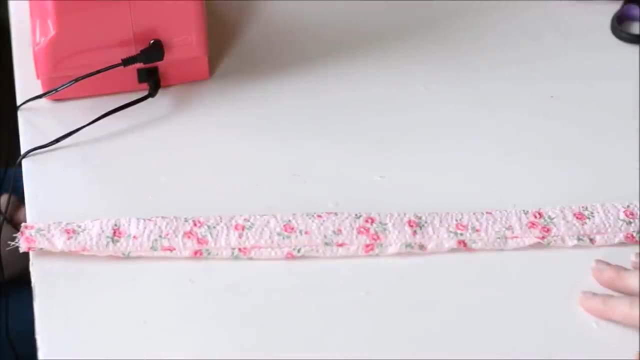 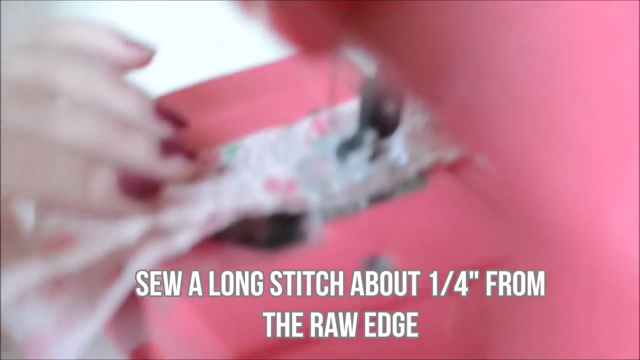 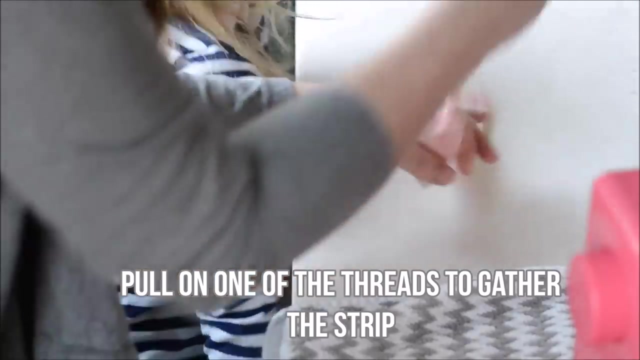 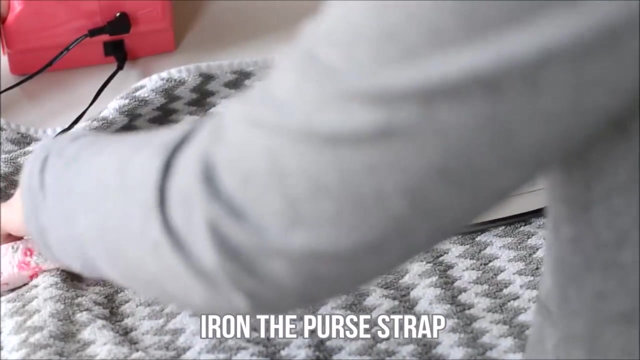 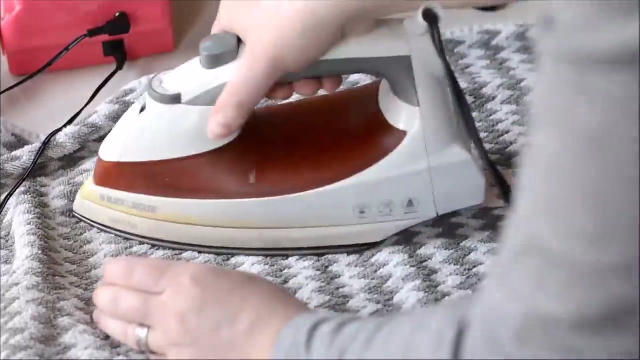 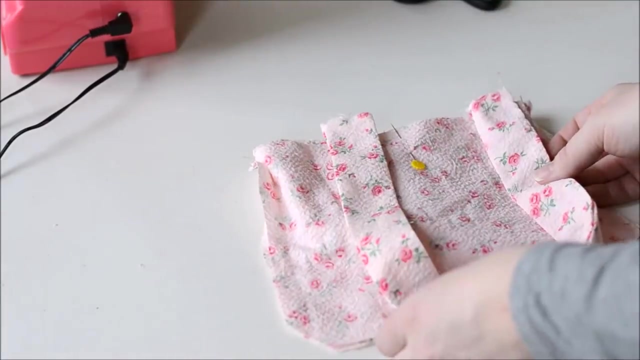 Now fold the third long strip in half lengthwise for the flower embellishment. Sew a long stitch about a quarter inch from the raw edge. Pull on one of the threads to gather the strip. Next you're going to iron the purse strap to make it nice and flat. 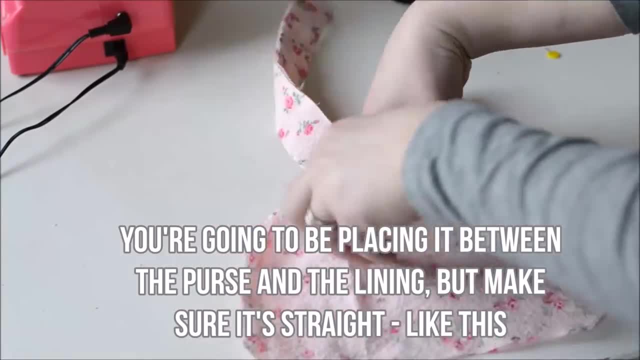 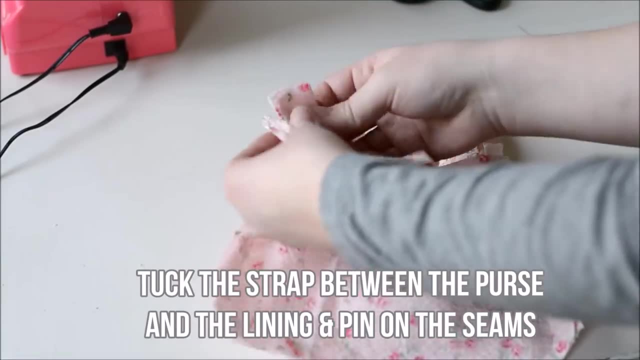 You're going to be placing it between the purse and the lining, but make sure it's straight, like this. Then tuck the strap between the purse and the lining and pin it onto the side seams like this. You're going to want to make sure it's straight, like this. 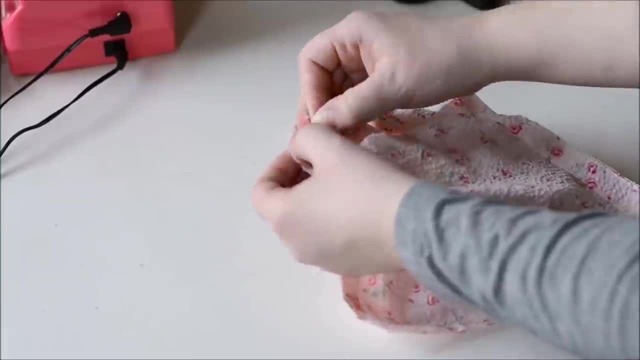 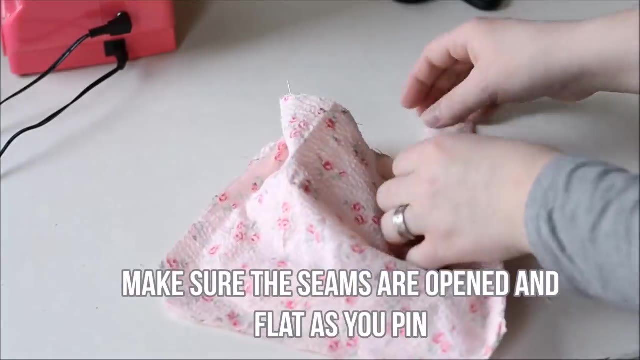 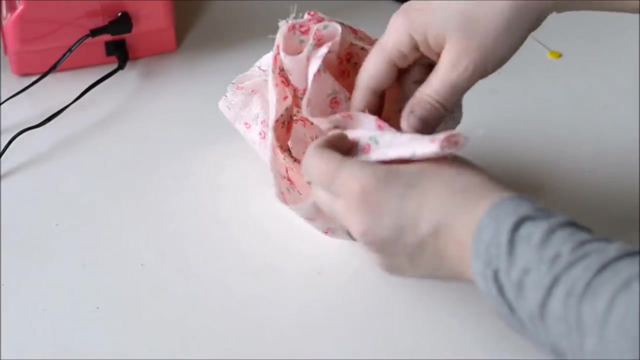 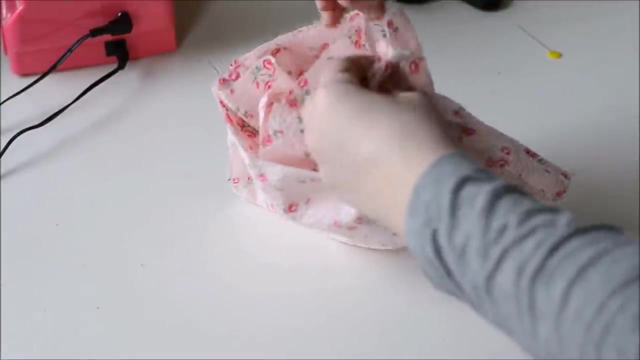 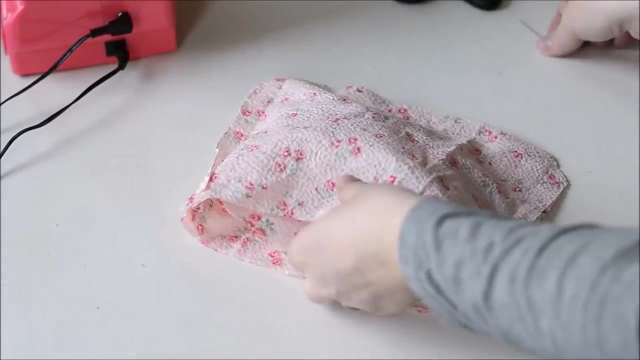 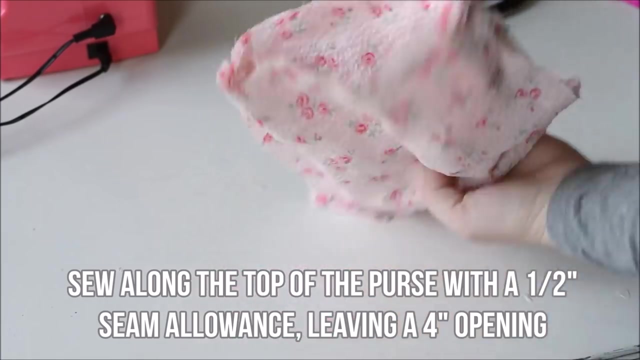 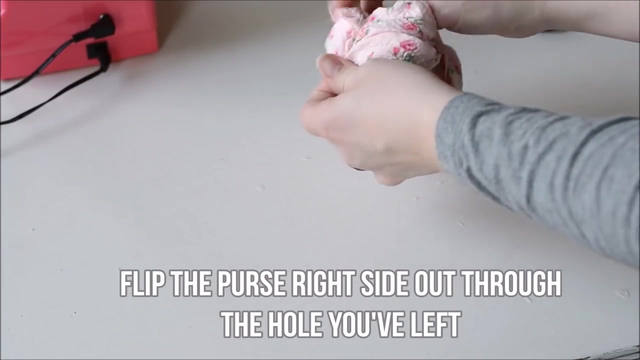 Make sure those side seams are opened up and flat as you pin. This will create a nice, smooth finish on the outside of your purse. Now sew along the top of the purse with a half inch seam allowance, leaving at least a four inch opening. Once you're finished that, flip the purse right side out through the hole that you left. 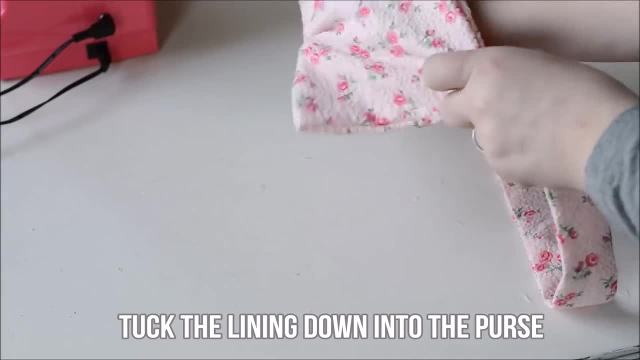 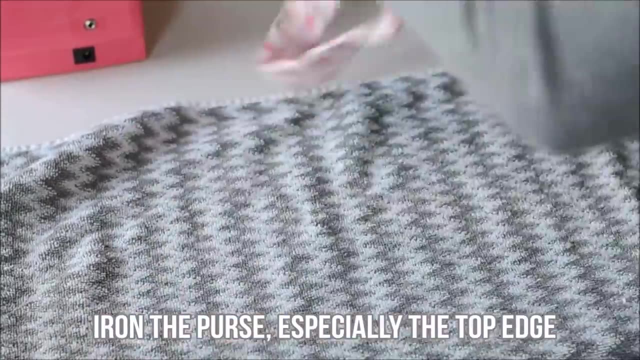 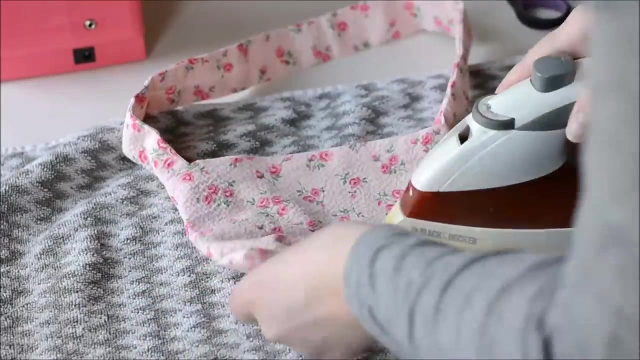 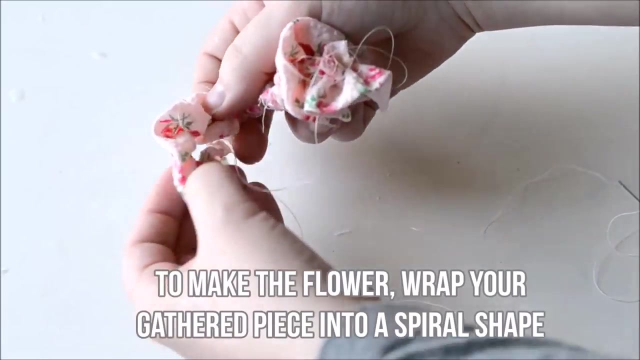 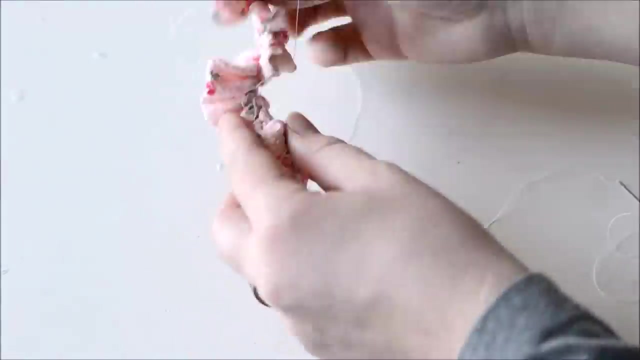 Now tuck that lining down into the purse. Iron the purse, especially that top edge, to make sure it's nice and flat. Now sew a quarter inch from the upper edge of the purse, sewing that hole shut To make the flower. wrap your gathered piece of fabric into a spiral shaped like this: 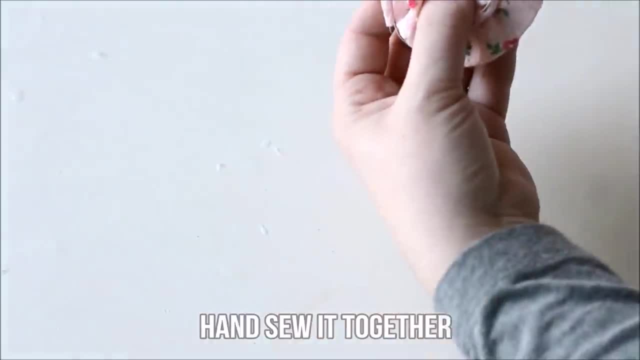 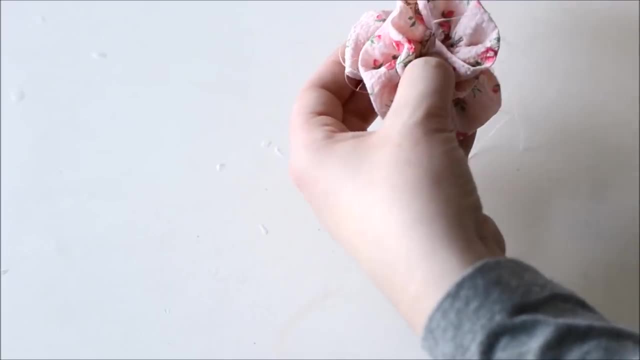 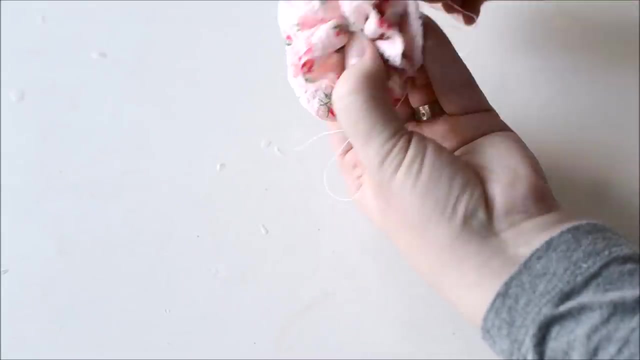 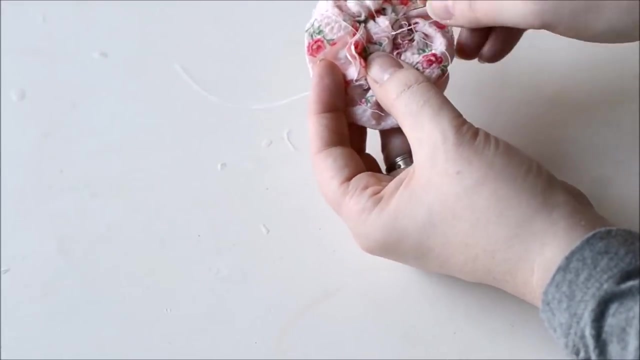 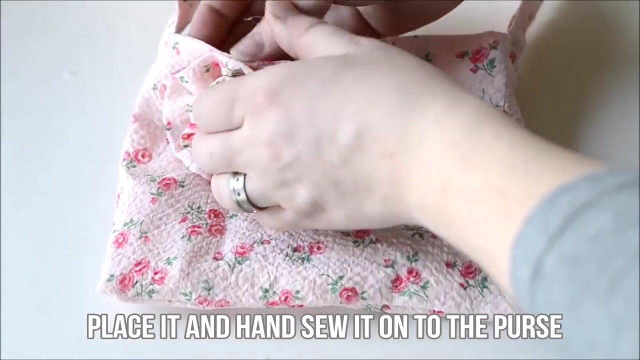 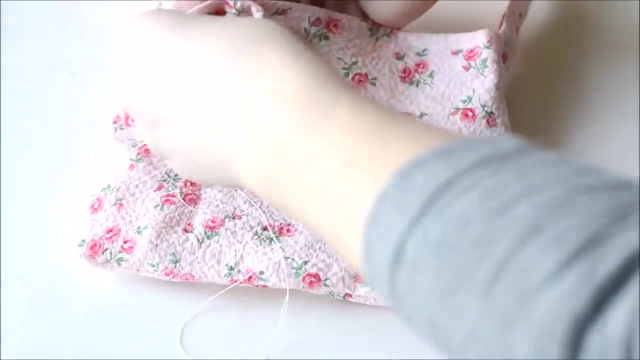 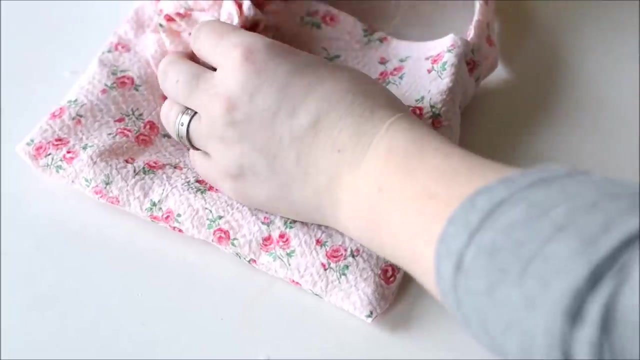 And sew it together to secure it. Put the flower where you want it to go- onto the purse- and hand sew it onto the purse. This can be another great project for your child if they want to try out hand sewing. So I'm basically just tacking it down every inch or so from the bottom edge of the purse. 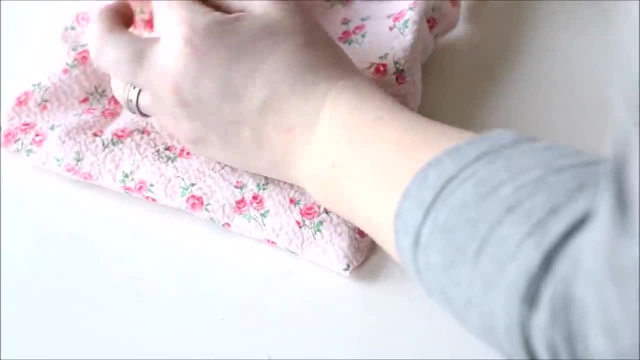 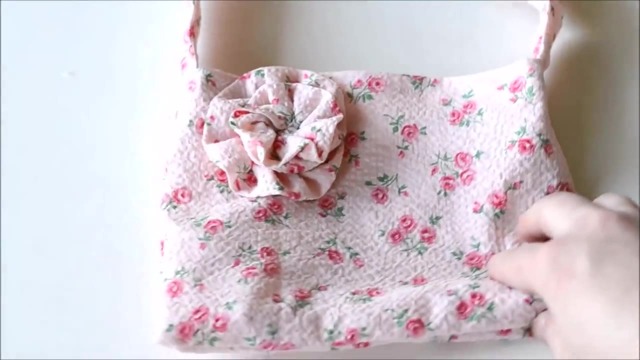 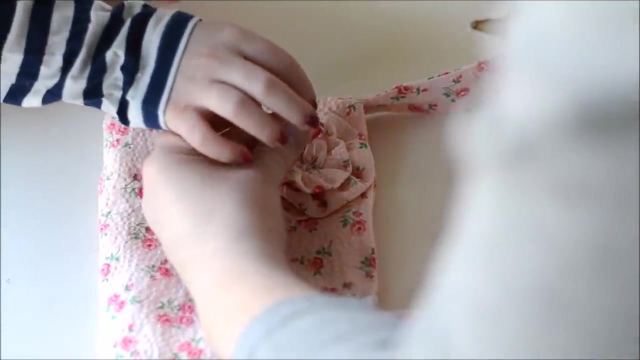 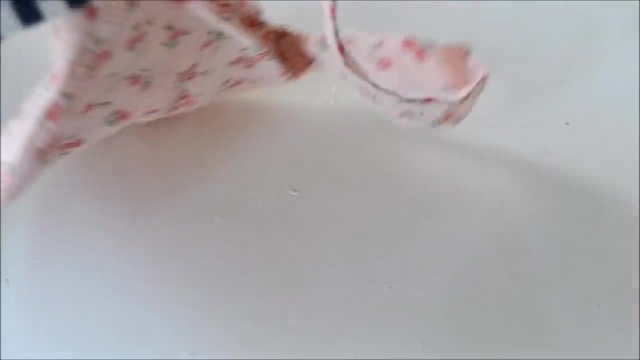 And finally, if you want to embellish the flower with a bead or a gem glued into the center, We just used a hot glue gun And that is it. You and your child have finished your beautiful purse. Like I mentioned, this is a fabric.